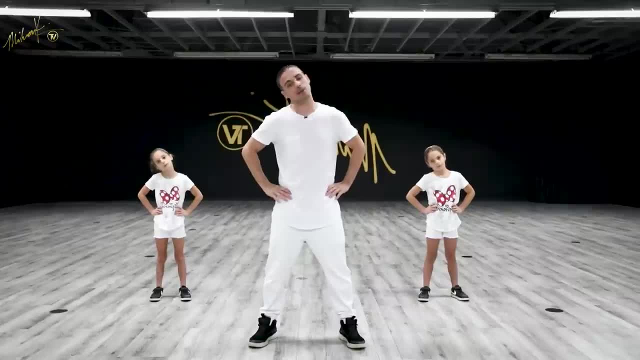 Take your time. One middle, two, middle, three, middle, four. Good, Switch, Go up. One middle, two, middle up, middle down- Good, Let's take the neck down. We're going to go over to the right side Circle around- Good, Now go to the other side Circle- Good, Awesome, Now the shoulders. We're going to bring it up on beat. We're going to go one drop, Two, three, four. Good, Let's go. 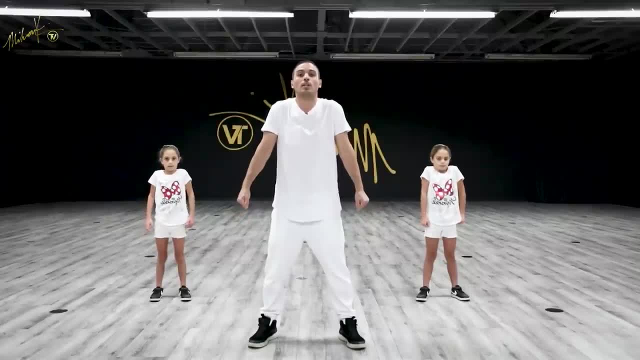 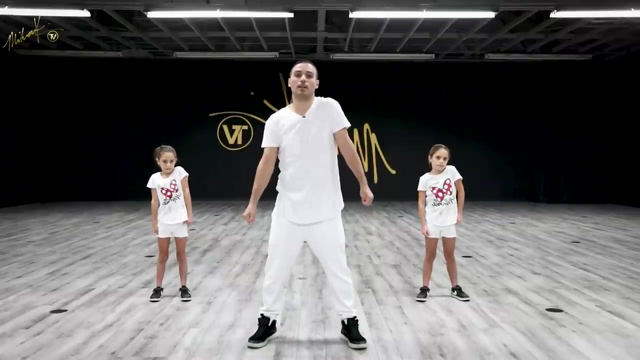 drop, three, drop four, drop, let's roll one- good, take your time. two and three, four, five, take it back slow. one, two, three, four, five, six, seven, let's speed it up. go one, two, three, take it back. and one, two, three, one by one, slow, right left, drop, drop again one, two, three, four. awesome guys, let's roll the. 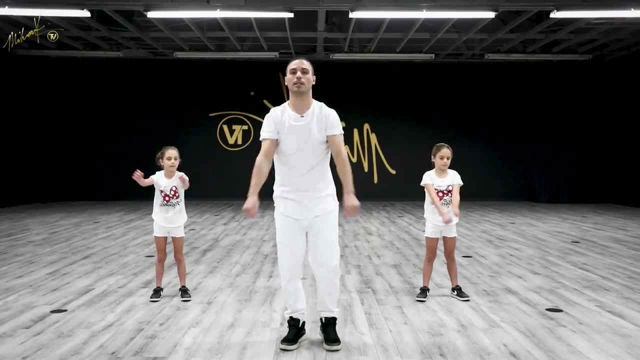 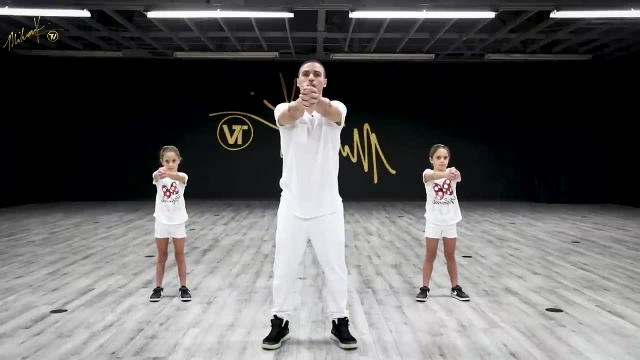 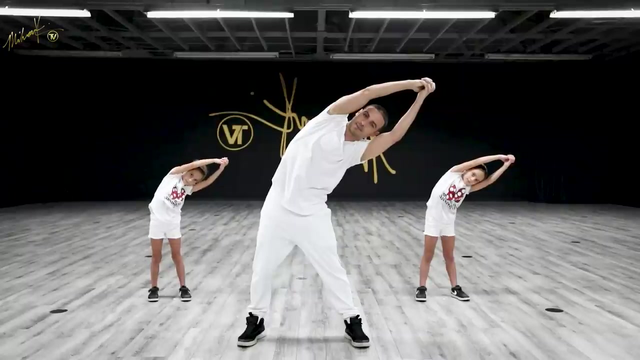 arms forward, big rolls, good, good. good, take it back. good, bring the arms out. hold your fingers and hands just like this. twist it out, stretch it out. good, flip it over again one more time. good, last time here, bring the arms up. we're gonna lean over and stretch it out. good, stay there. good. good. good, slowly take it to the other side. 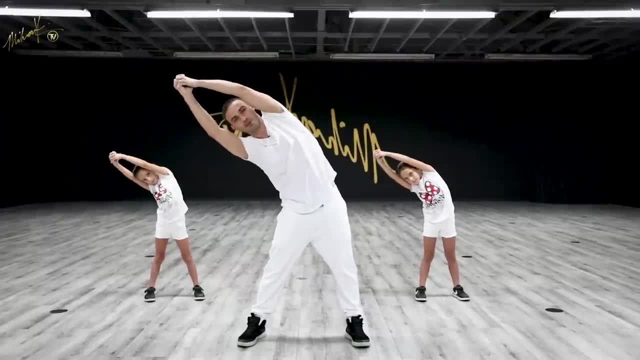 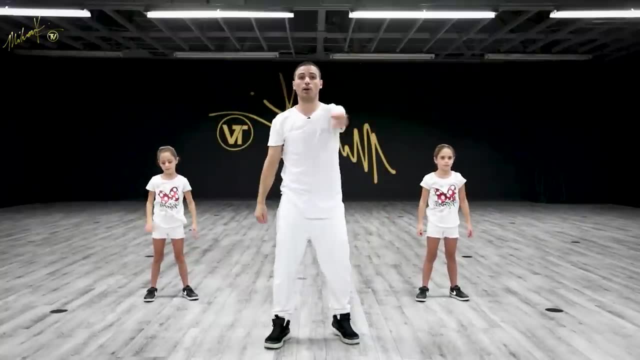 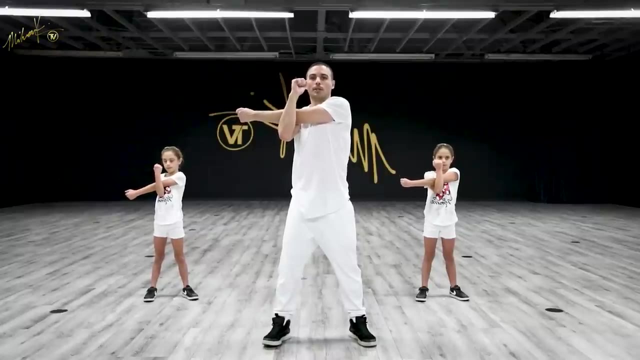 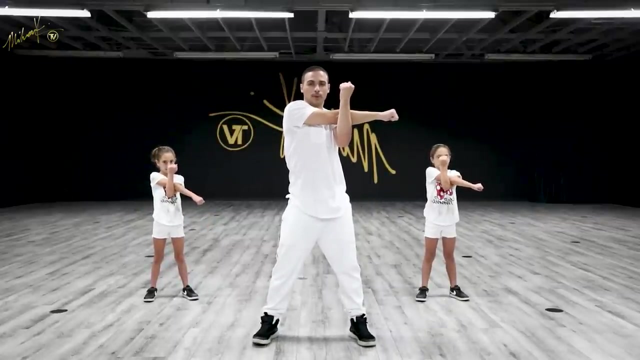 keep your hands above your head. keep your hands straight, too. awesome, come on out. take the arms out. let's bring the right arm. cross it in front, left arm underneath. good, let's hold this. good, switch the arms here we go. good, all right, release. let's bring the arm up. it's gonna go behind your back. 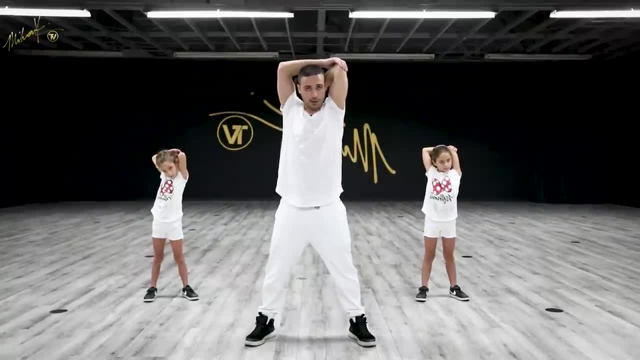 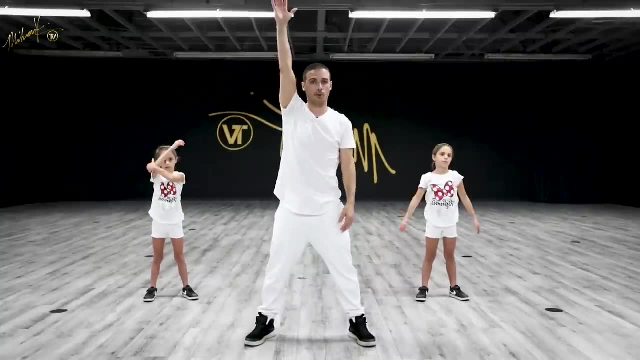 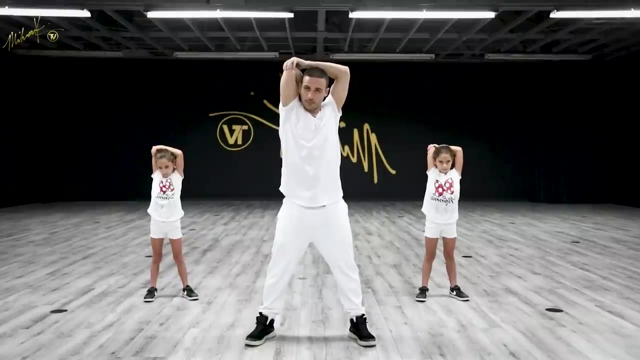 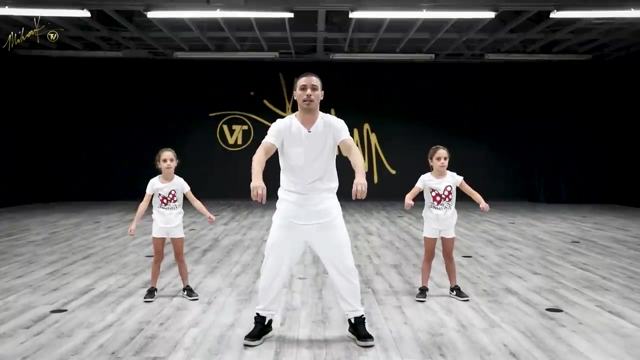 bring the other arm up. pull it in. good, let's hold that for a couple of counts. good, awesome, switch the arms. here we go. whoop up- good, hold that. awesome guys, release now your body. we're gonna push the chest forward out. hold it. take it back- good, again. front and back one more time. here we go. 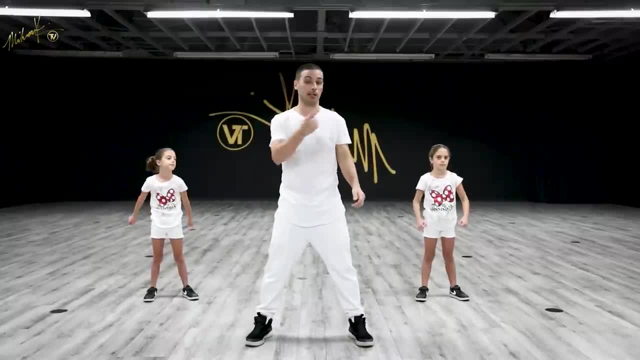 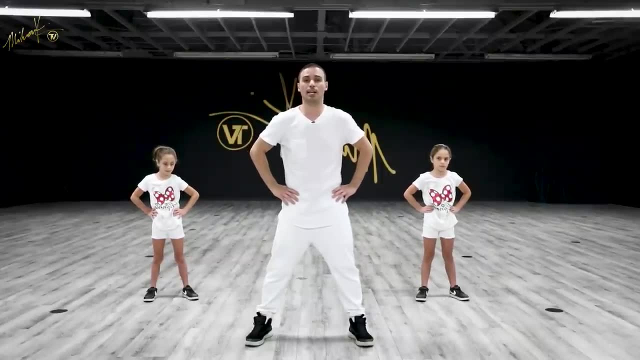 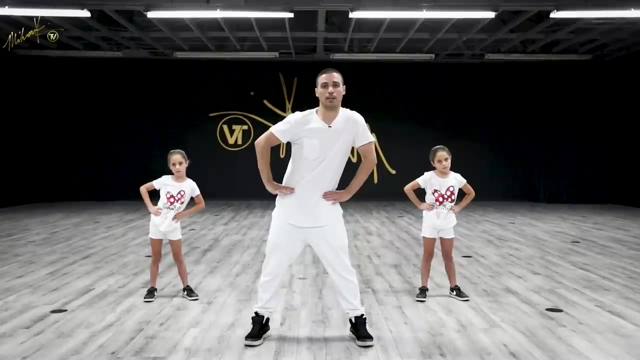 front and back. good, now we're going to get side to side. this one gets a little tricky. let's put the hands on the hips. make sure it's your body moving and not your hips. here we go. five, six, seven, over to the right. here we go. this is one, hold it there. two, good again. three, four, keep going. 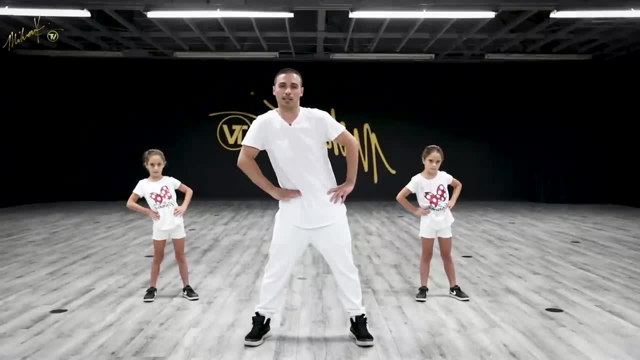 couple more times. five: i know this one should be more difficult to do. keep going, keep going. five: i know this one should be more difficult to do. it's tricky, it's okay, just try it. seven: good, eight, awesome. now we're going to go. 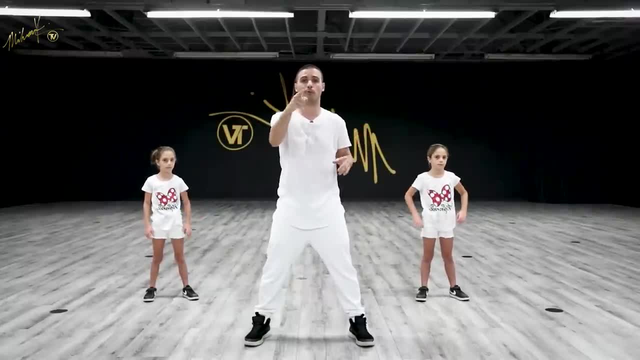 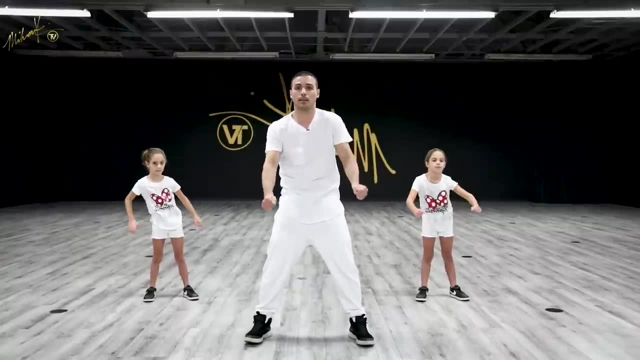 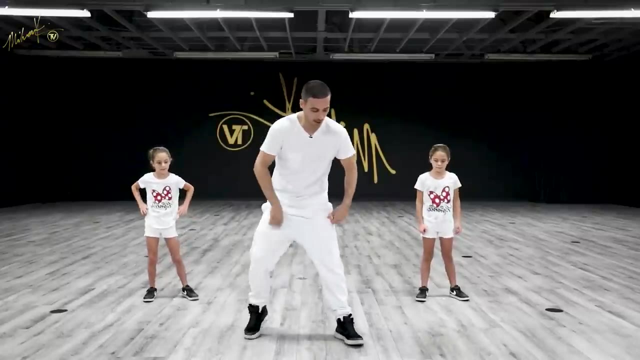 across. we're going to go forward right back left, and then we'll repeat: forward left back right. here we go ready, girl six, seven, eight. forward right back left, switch forward, left back right. good, alright, let's go down to the legs. now keep. 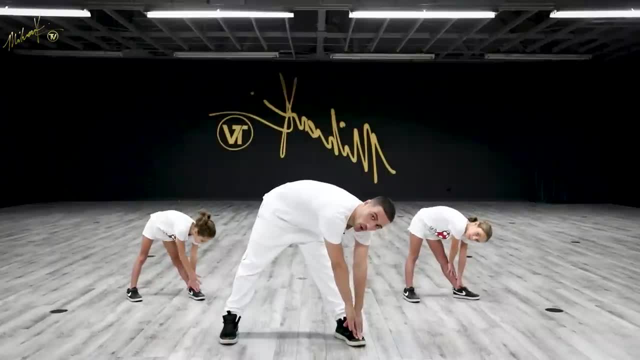 the legs straight. just reach down and touch your toes if you can. the goal is to keep the knees straight. okay, if you have to bend the knees, then just go as far as you can go. once you feel good with that, let's go to the middle hands down to the floor. 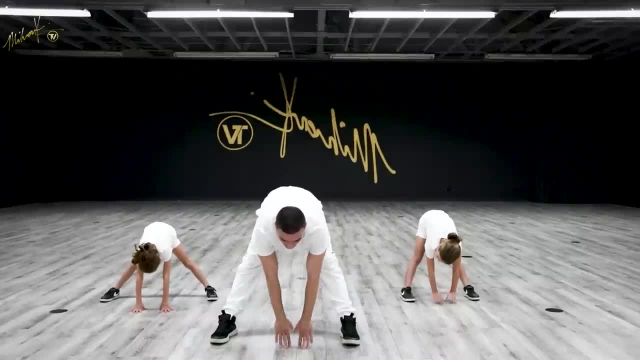 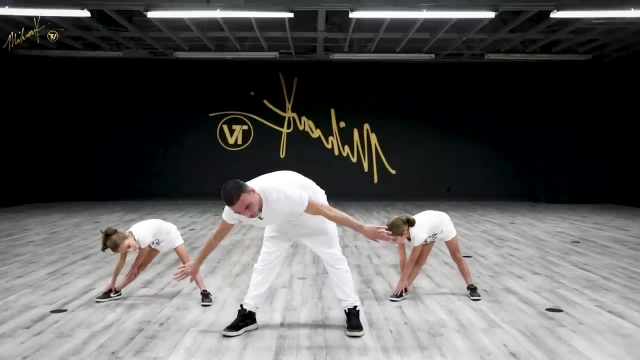 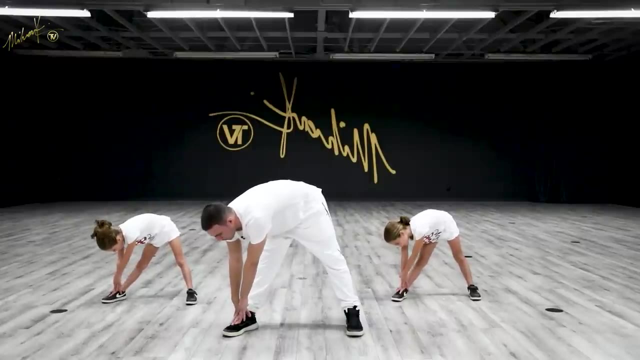 if you can again, knees are staying straight. good, good, good, perfect. let's switch now to the left leg. here we go. you don't need to go too wide, just shoulder length. yeah, here we go. alright, perfect, bring the legs together. 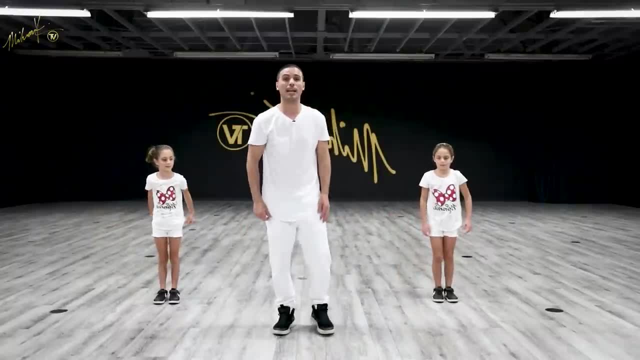 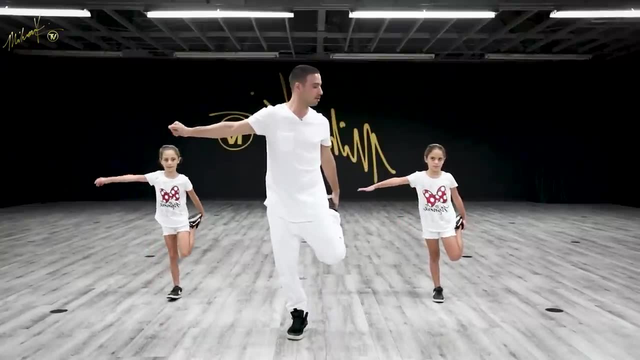 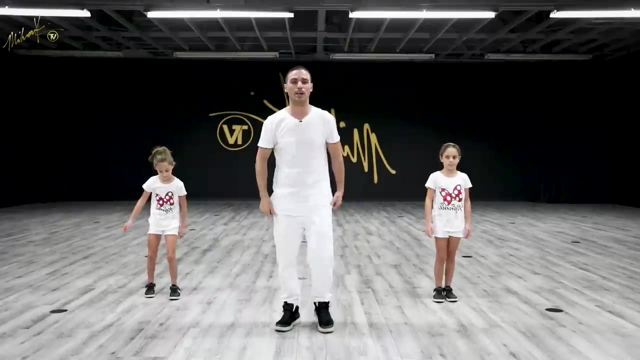 kick them out, kick them out, kick them out. let's bring the right leg up and hold it for eight counts. girls, you ready, here we go and hold your balance: two, three, four, five, six, seven, eight, awesome, let's switch the legs. it's okay if you lose your balance. 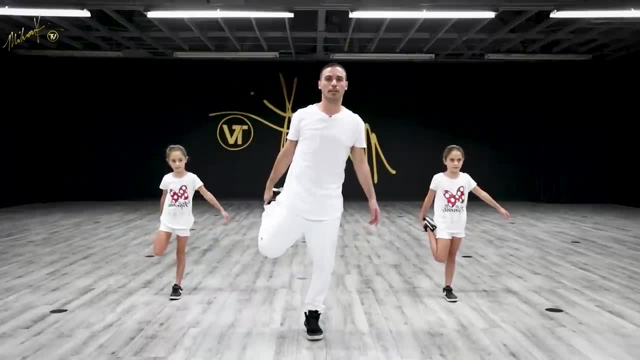 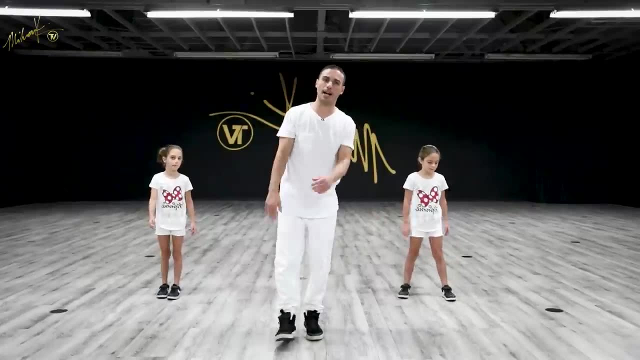 just get back at it. okay, here we go. another eight counts: one, two, three, four, five, six, seven, eight, awesome, alright, we're gonna go right into our jumping jacks now. we're gonna do eight to the front, eight to the. 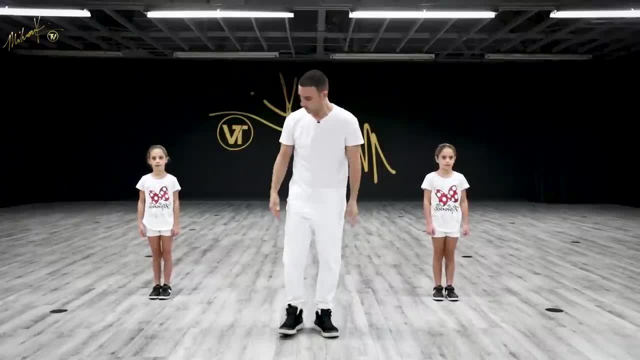 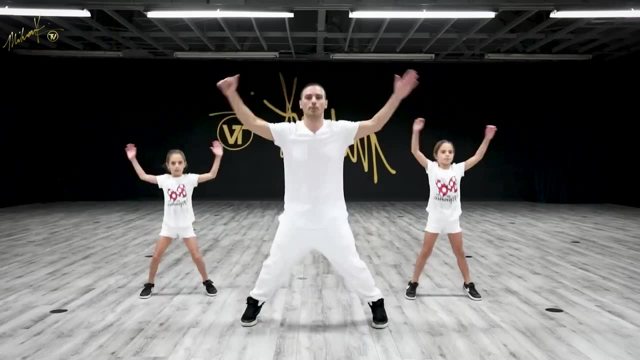 side back to the front and eight to the side. here we go, feet together, girls, you ready, and five, six, seven let's go, and one, two, three, four, five, six, seven and switch one. 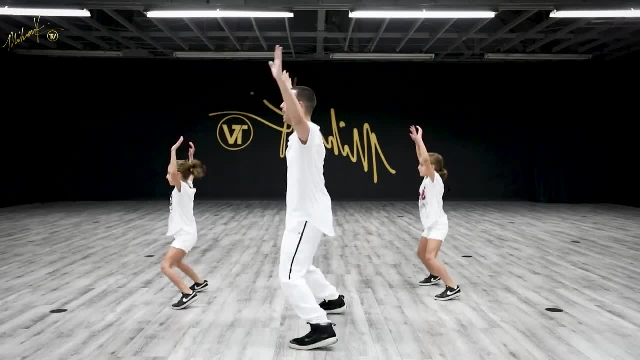 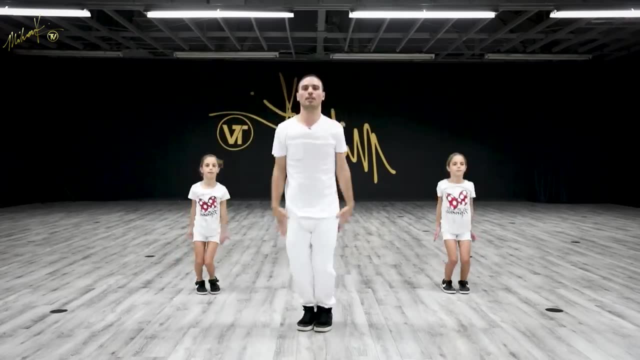 two, three, four, five, six. we're gonna come back to the front, here we go: switch one, two, three, four, five, six. now we're going over to the right, here we go, and one, two, three. 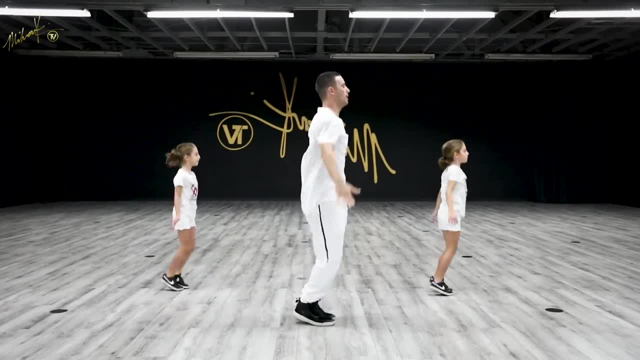 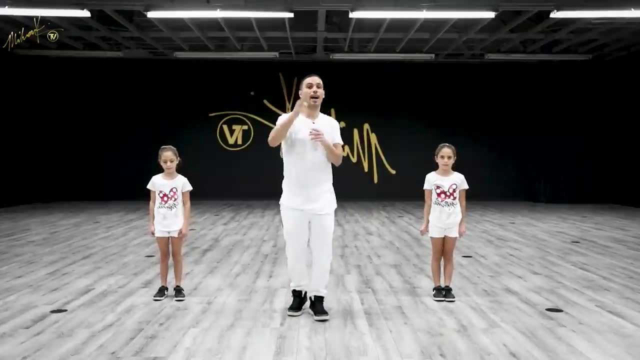 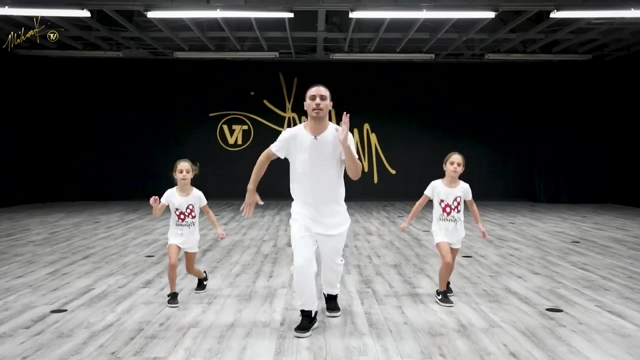 four, five, six, seven, eight. good, next one is gonna be the scissor kicks. okay, five, starting with the right leg. five, six, seven. go one, two, three, four, five, six, seven. 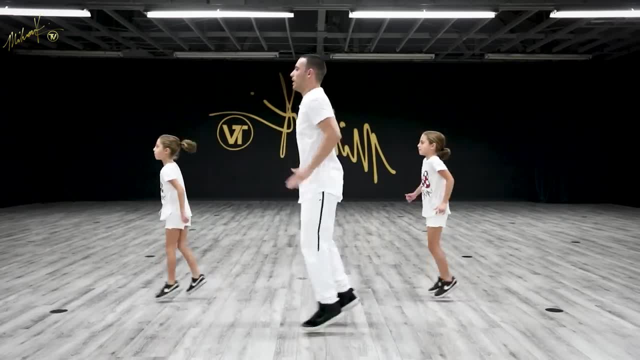 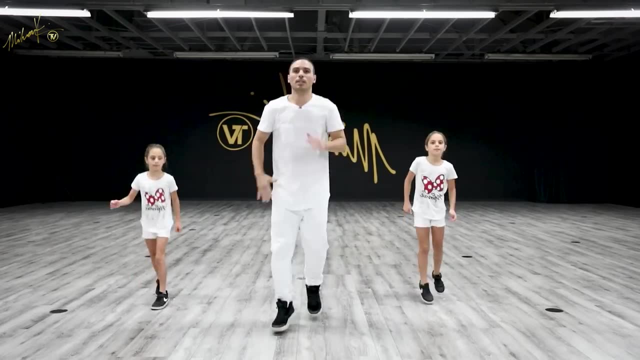 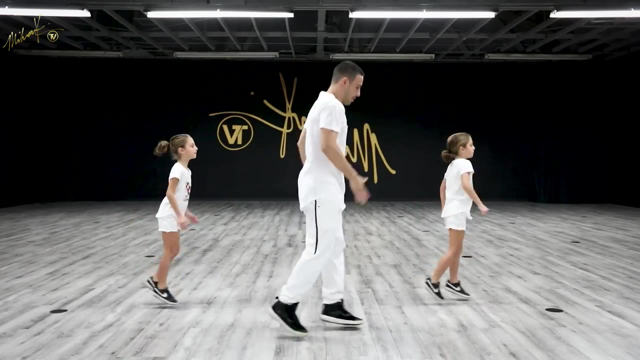 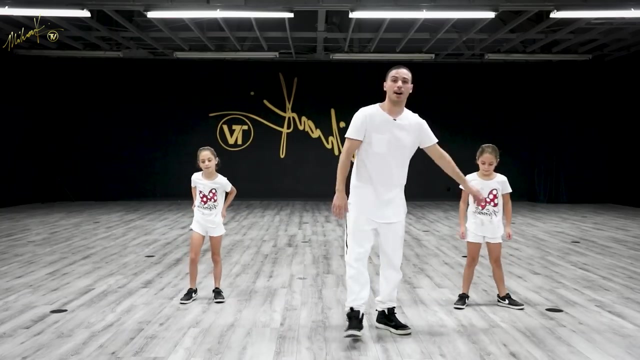 eight switch. one, two, three, four, five, six, seven, eight switch one, two, three, four, five. you can use your arms if you want seven switch and one, two, three, four, five, six, seven, eight. good, alright. 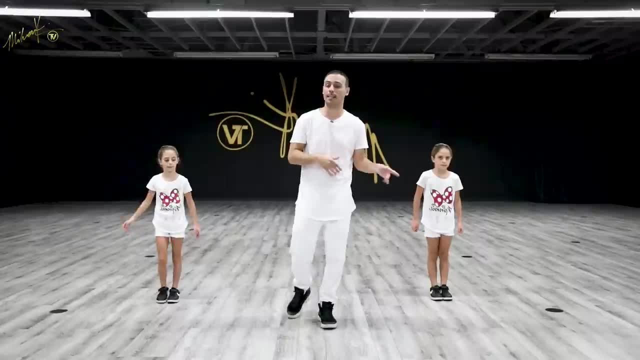 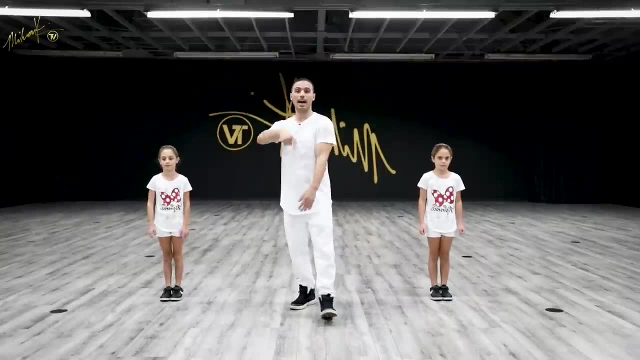 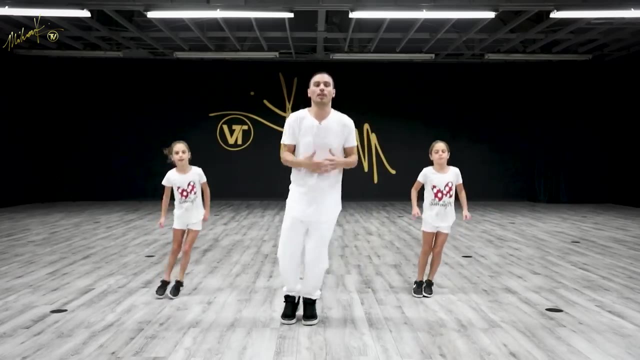 we got one more left feet together. we're just gonna go side to side. okay, give you a second to breathe. ready, ladies, last one, here we go, and five, six, five, six, seven. go one, two, three, four, five, six. 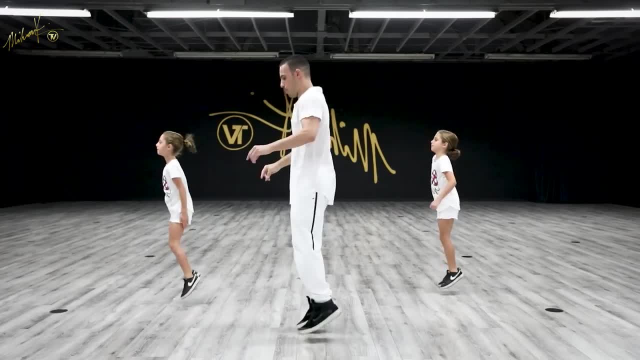 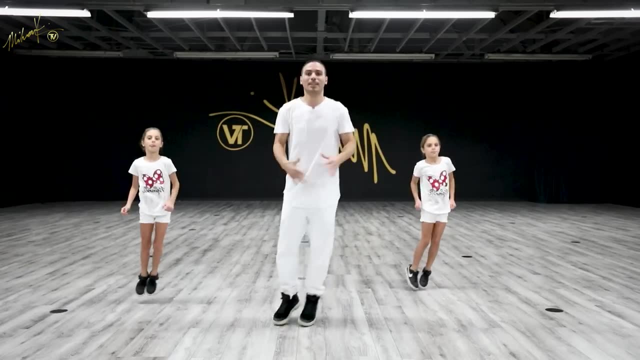 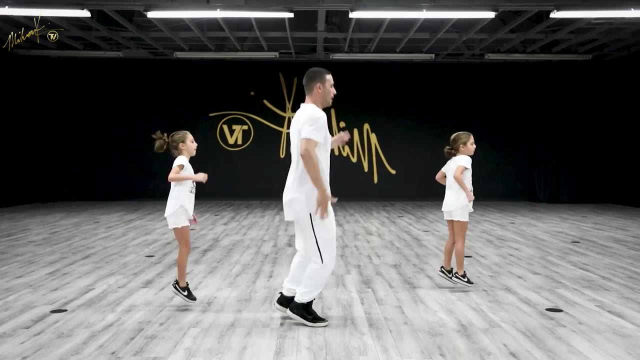 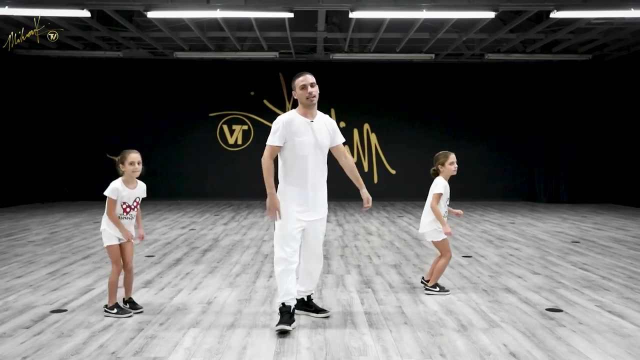 seven. switch one, two, three, four, five, six, seven. back to the front, let's go one, two, three, four, five, six, seven. last eight. here we go one, two, three, four, five, six, seven, eight. awesome guys, let's get ready to dance.